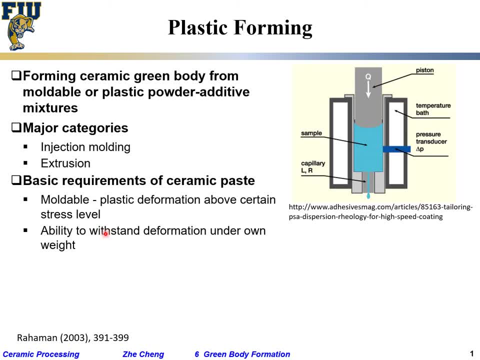 into a container, hold it before it dries here. once you release it from the mold, well, you pretty much have the same stuff, but it has to be able to maintain roughly its shape without collapsing, without significant plastic deformation. okay, extrusion instrument: people talk about a piston type. 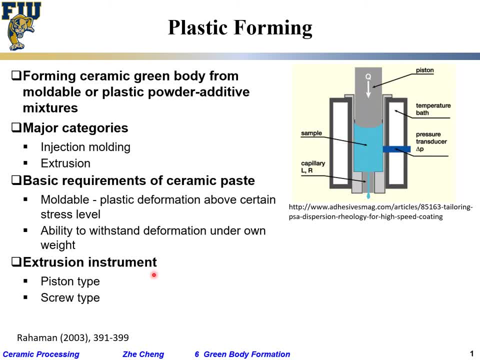 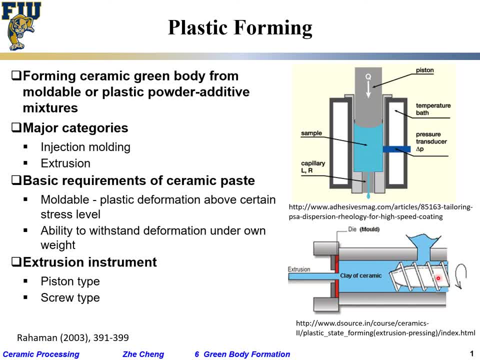 screw type or screw type. using a screw type, using a screw type, using a screw kind of machine, something like this: you are adding feed to here and this is your so-called screw and it rotates and pushing the paste, thick ceramic paste, through here, through a. 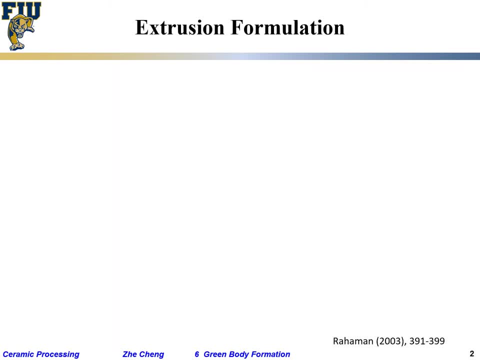 opening with certain shape extrusion formulation. the formulation is very important to manipulate the plastic behavior, like how we whiskers. it's going to be what's the so-called yield strength right? how much shear stress it can withstand before it's plastically deformed? for clay it's. 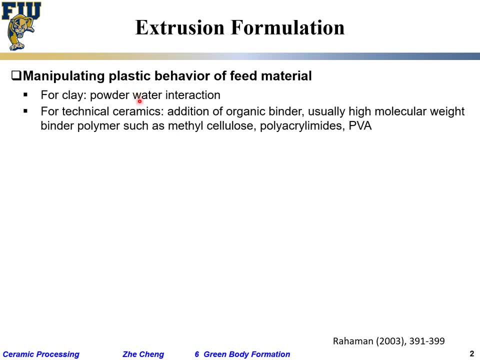 related to powder-water interaction and for technical ceramics. quite often people add organic binder. how much organic binder? what types of organic binder and what's the molecular weight of the organic binder people are adding in? and what's the so-called plasticizer right to reduce the TG? 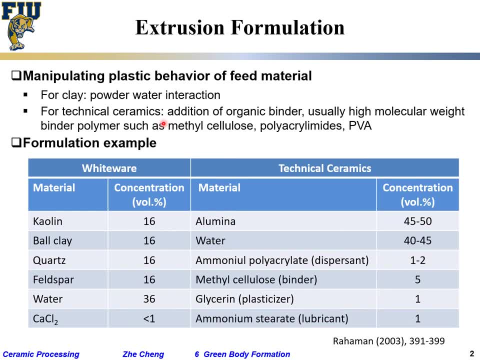 to allow it to flow, and a formulation example. here I'm giving two types. one is so-called white wire. where do we use white wire? toilet, typical toilet, white wire washing basin, something like that- and quite often you have a formulation. 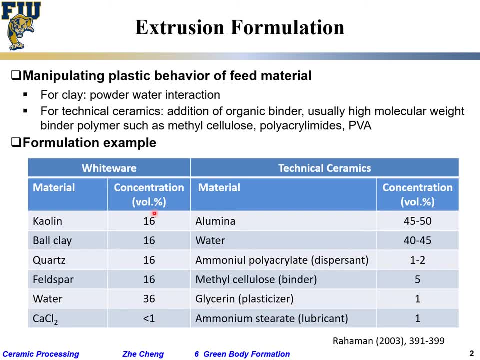 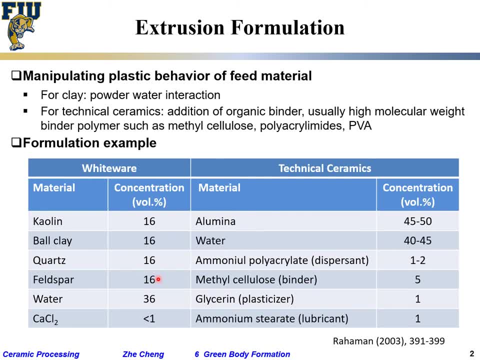 ceramic phase. different ceramic phase give it a different property and a lot of details into it. I'm not even expert, but anyway complex for technical ceramics. for example, people are trying to make high purity aluminum oxide. okay, 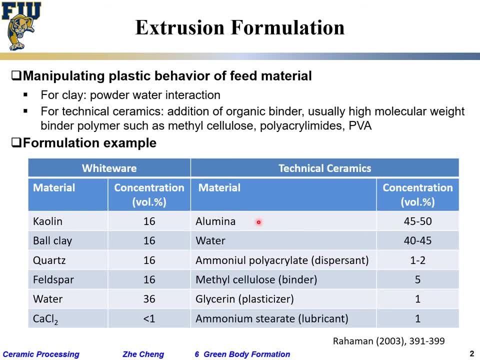 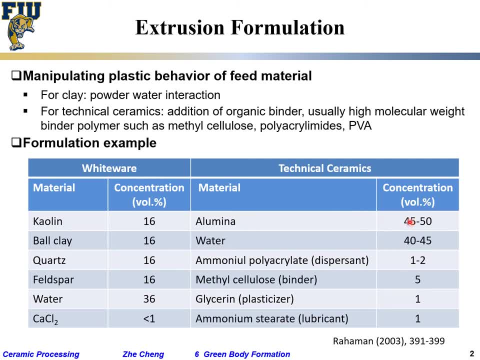 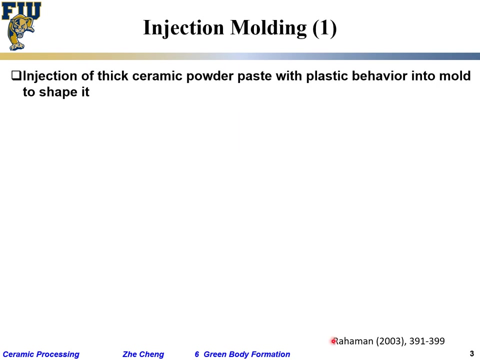 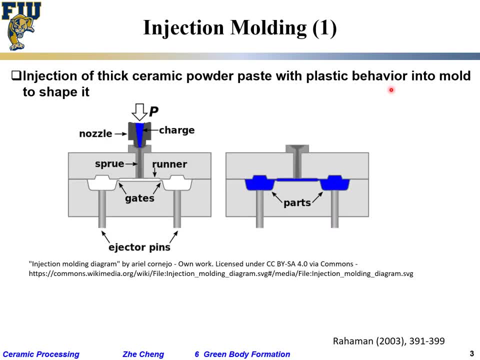 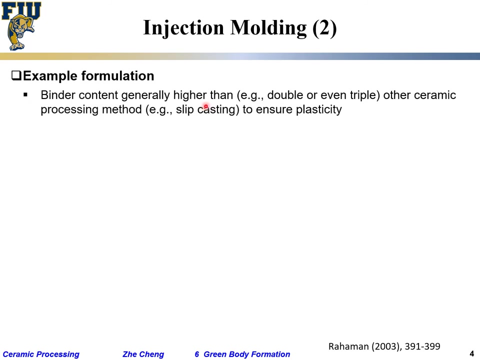 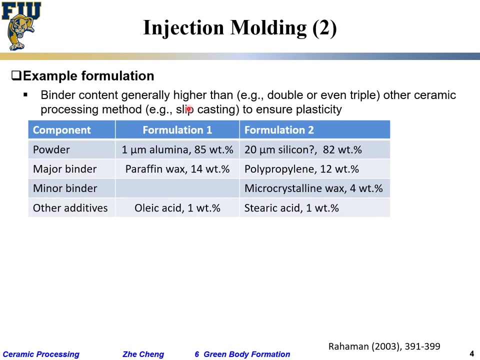 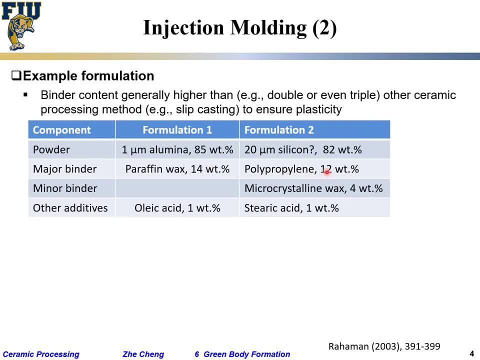 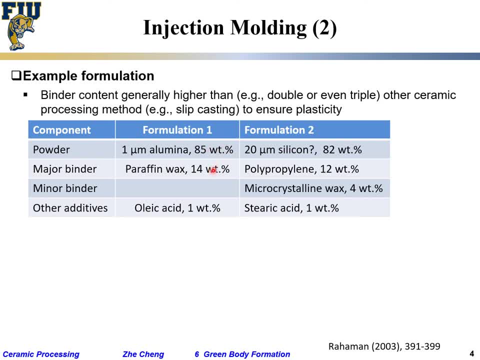 density. well, it means it has a lot of volume. this typically has higher density, right one, two, five, and the density let's say is two to one or three to one. by volume actually can be around two to one, three to one. by volume it's a lot of polymer bundle- okay, and some other additives, injection. 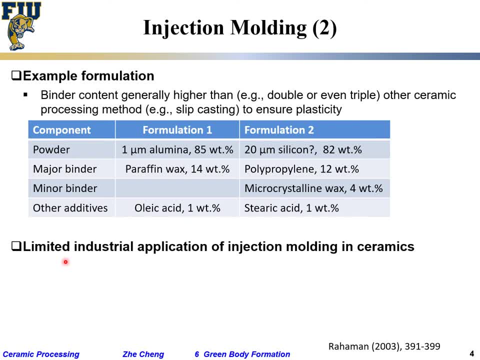 moldings actually have not a broad industry application because tooling cost. tooling cost can be expensive unless you are really going to very high volume production. otherwise typically a precision mold cost tens of thousands of dollars or even more expensive. and that high polymer content- all these 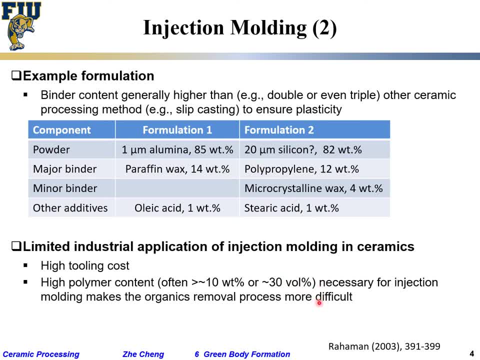 are necessary to remove them, but they are pretty difficult if your polymer content is high. and do you imagine when you remove polymer, the polymer, if you burn them, polymer becomes carbon dioxide and the water those escape as gas and you have difficulty to maintain it if you do. 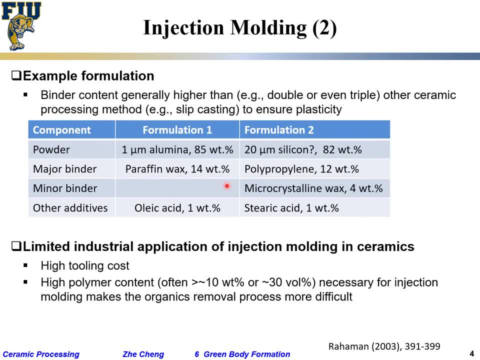 them too quickly, it's going to have a so-called explosion right the too much bubble gas formation, you are going to explode your body. so that's why high polymer content, which is tricky or difficult for you to remove. that's why injection molding: you mold it. you need a lot of plastics or polymer, but you have to be very 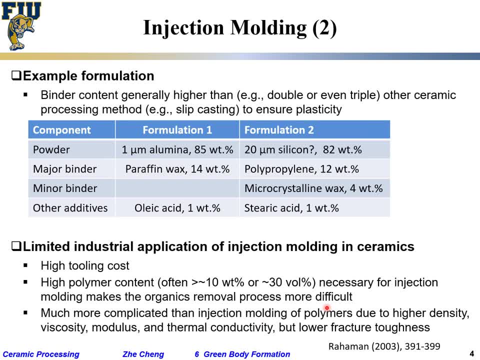 careful with bundle removal, okay, which limits its application. it's uh more complicated than injection molding of what polymer people do. injection molding of polymer, pure polymer, a lot, and it's cheap, very, very cheap. but for ceramic paste, although it still has that plasticity, it's way more difficult to do than 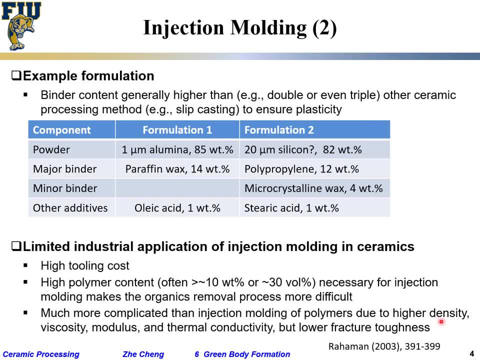 polymer, because the plastic, the ceramic paste, compared with polymer, has much higher density. polymer the density is quite often only around one, slightly higher than one. ceramics, depending on the whaticanic you are dealing with, can be much higher, much higher with viscosity, which means it's having difficulty. you need a higher pressure. 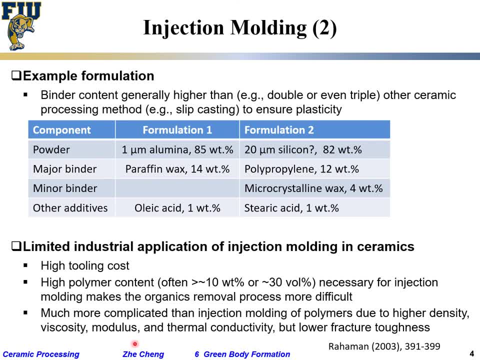 to penetrate into fine shapes, much higher modulus. you're talking about the composites. the modulus is the contribution for the polymer part plus the modulus for the ceramic part, which can be tons, or which can be tons or hundreds times higher than the polymer you are dealing with. make sense, which means, if you want it to be, 있는데요.